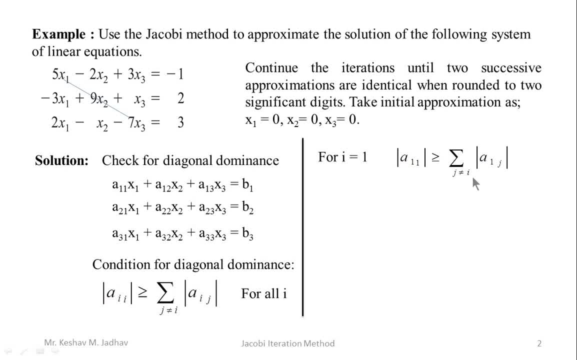 For j is not equal to i, For j is not equal to i. So here a11 is 5.. So absolute value of 5 should be greater than or equal to summation of absolute value of minus 2 and absolute value of 3.. 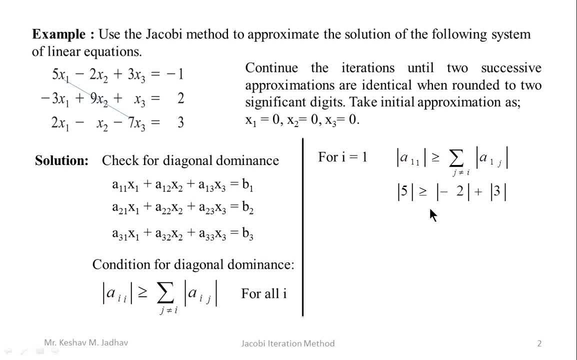 So here this: 2 plus 3 is 5.. So it is equal. So this condition is satisfied. Then, for i is equal to 2,. we can rewrite this equation like this: Here this a32 means 0.. 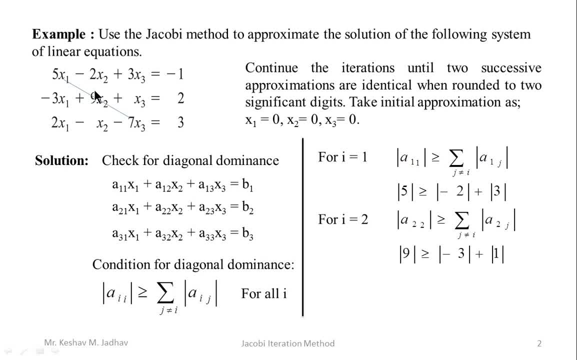 And here this الظ equal to1i, And here this сл is equal to 1. is 9.. So absolute value of 9 should be greater than or equal to summation of absolute value of minus 3 and absolute value of 1.. Here this 3 plus 1, it is 4.. So 9 is greater than. 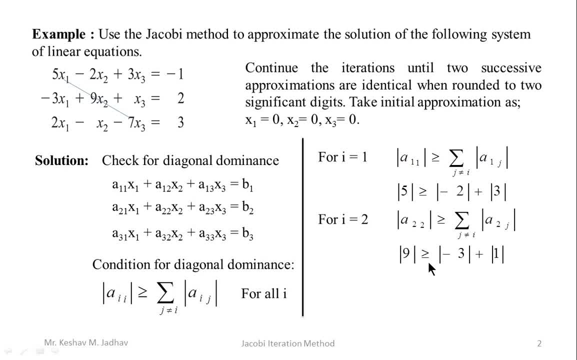 4. So for i is equal to 2. also, this dominance character is satisfied. Now, for i is equal to 3, if we put i is equal to 3, then we will get this condition Here. this 833 means minus. 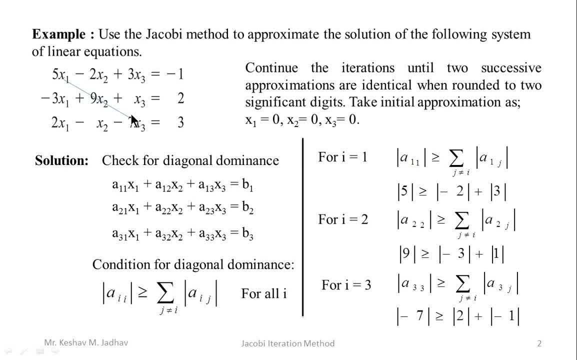 7.. So here this absolute value of minus 7 should be greater than or equal to absolute value of 2 and absolute value of minus 1.. So here, absolute value of 2 plus absolute value of minus 1, it is 3.. And absolute value of minus 7 is plus 7.. So this 7 is greater. 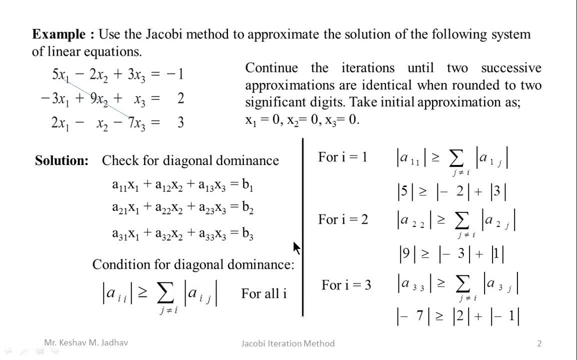 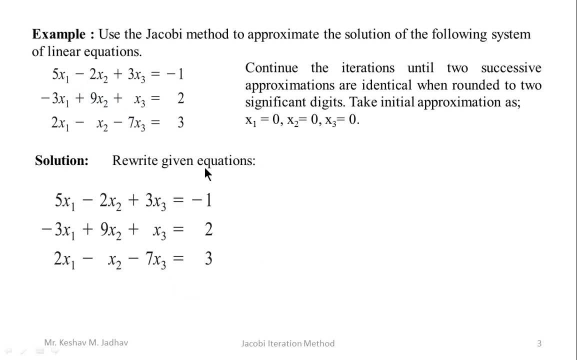 than 3.. So here condition for diagonal dominance is satisfied. So it is not required to rearrange the equations. So as this condition is satisfied, we can go on. So for next step of Jacobi iteration method. So here we can rewrite this equation From: 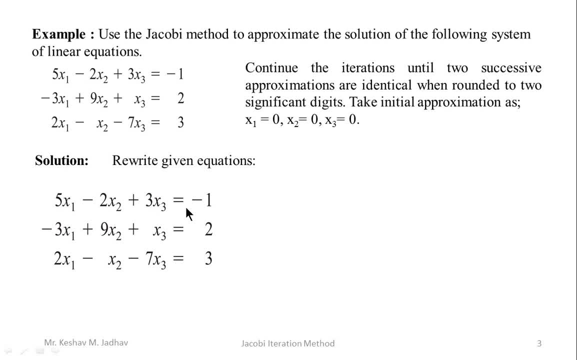 first equation we have to take x1 on one side and remaining terms on another side of equal to sign. From second equation we have to take x1 on one side of equal to sign and all other terms on another side of equal to sign. And from third equation we have to: 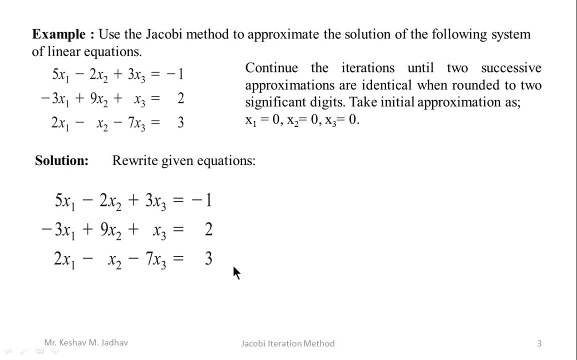 take x3 on one side and all other terms on another side of equal to sign. So we can rewrite this equation like this: From first equation we have taken here X1 on one side and remaining terms on another side of equal to sign. So here we will get formula for x1.. From second equation, if you. 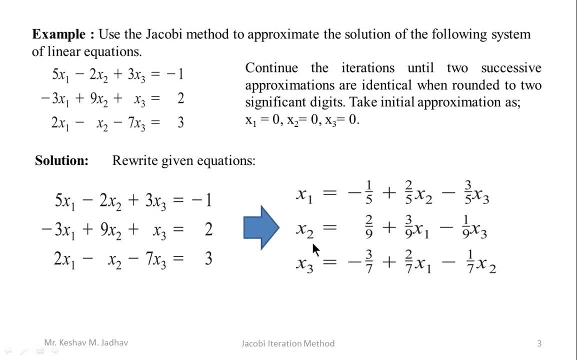 take x2 on one side and all other terms on another side of equal to sign, then we will get formula for X2.. And from third equation, if we take X3 on one side of equal to sign and all other terms on another side of equal to sign, then here we will get formula for. 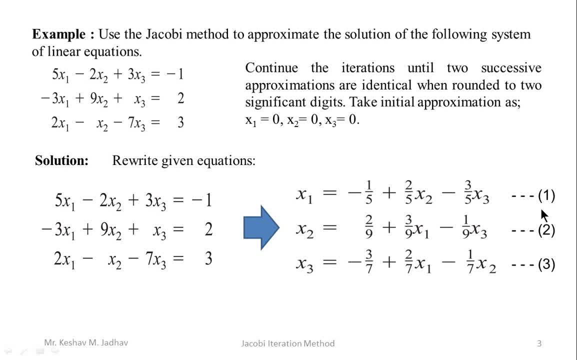 X3. So here we can give the equation number, Equation NO.1, equation NO2.. Division helps equation number 2 and equation number 3.. Now these equations will act as the formula for calculating values of x1, x2, x3.. So let us start iteration number 1.. Now, as given in, 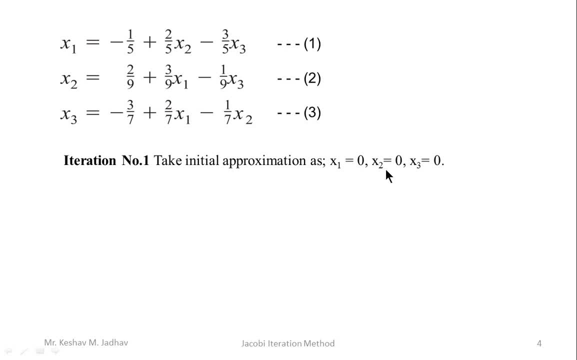 problem. we have to take initial upper animation, as x1 is equal to 0, x2 is equal to 0 and x3 is equal to 0.. If you put these values in these equations, then we will get next upper animated value of x1, x2, x3.. So let us put these values in these equations. So. 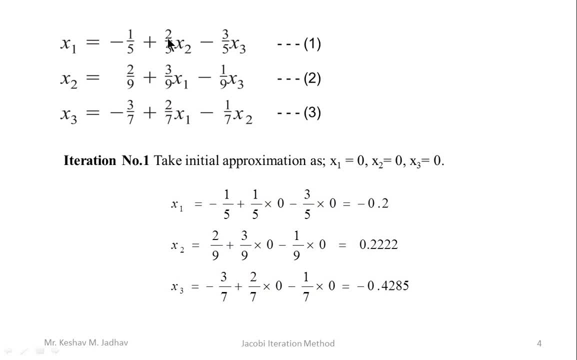 here we can see: x1 is equal to minus 1 by 5 plus 2 by 5, and value of x2 by 0 minus 3 by 5 into value of x3 is 0. So if you put the values of x2 and x3, then we will get. 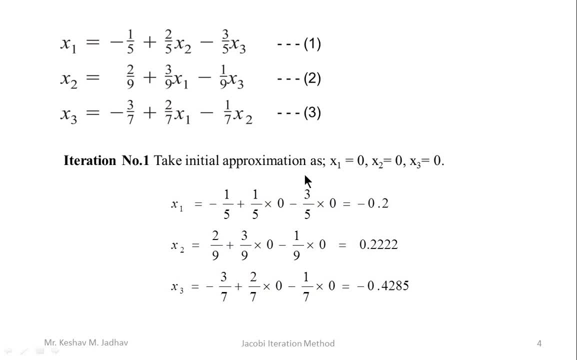 new value of x1 as minus 0.2.. Now if you put these values in equation number 2, then here we will get values of x2.. So x2 is equal to 2 by 9 plus 3 by 9. into value of x1 is 0 minus 1 by 9. into value of x3 is: 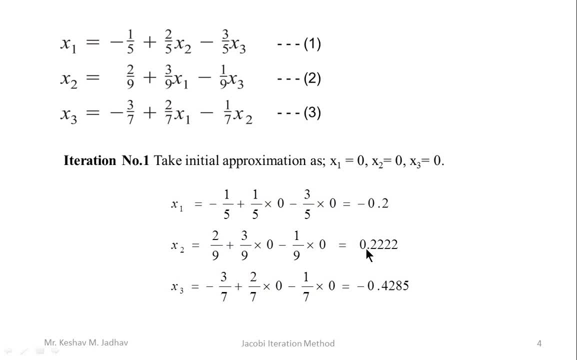 0. So here we will get new value of x2 as 0.2222.. Then if you put these values of x1, x2, x3 in third equation, then we will get new value of x3. So here x3 is equal to minus 3 by 7, plus 2 by 7. 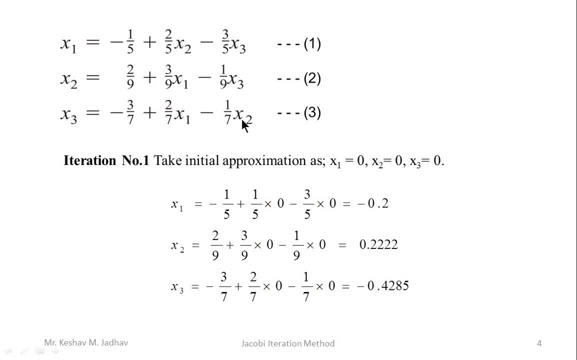 into: value of x1 is 0 minus 1, by 7, the value of x2 is 0.. So by putting value of x1 and x2, we will get new value of x3 as minus 0.4285.. So by putting x1 is equal to 0, x2 is equal to 0 and 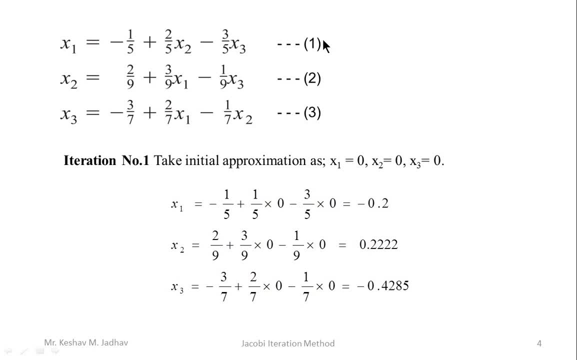 x3 is equal to 0. in these equations we will get new value of x1, x2, x3.. So these are the new approachability value for x1, x2, x3.. Now we will go for second iteration. 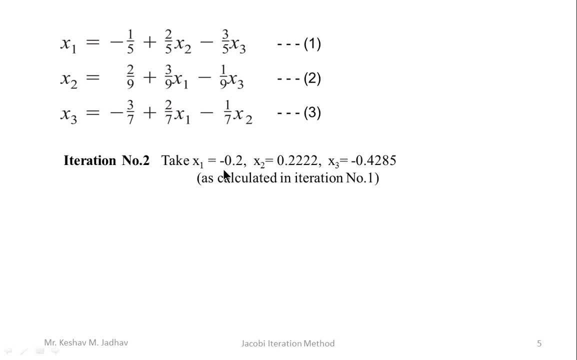 So for iteration number 2, we have to take x1 as minus 0.2,, x2 as 0.2222 and x3 as minus 0.4285.. These values are calculated in iteration number 1.. So here we have to repeat the procedure. 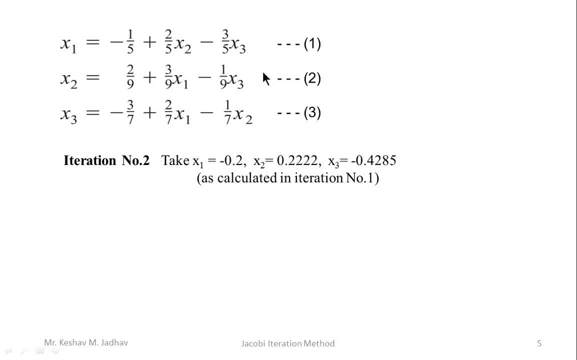 So here we have to put these values of x1, x2, x3 in these equations so that we will get next approximation for x1, x2, x3.. So here for equation number 1, x1 is equal to this, minus 1 by 5. as it is plus 2 by 5 as it is into value of x2, it is 0.2222. 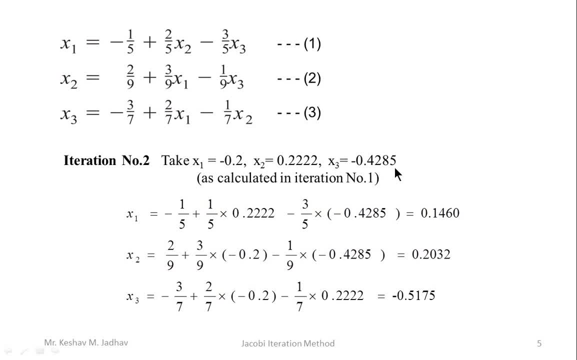 Minus 3 by 5 into value of x3 is minus 0.4285.. So if you put these values, then we will get new value of x1 as 0.1460.. Then for second equation, x2 is equal to 2 by 9 plus. 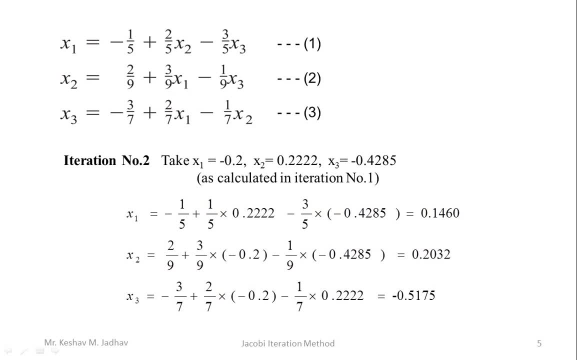 3 by 9 into value of x1. So we have to use value of x1, which is calculated in iteration number 1.. So value of x1 is minus 0.2.. Don't use new value of x1. We have to use values which are. 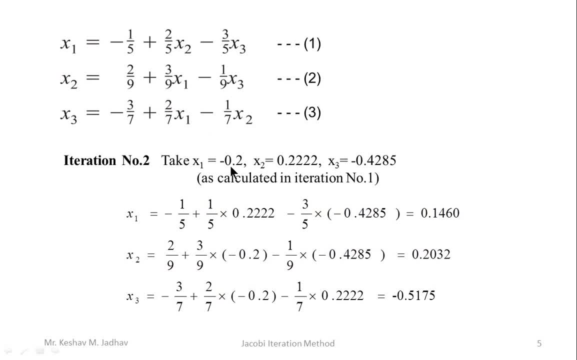 calculated in previous iteration. So here value of x1 is minus 0.2.. Then minus 1 by 9 into x3. So here x3 is equal to minus 0.4285.. So if you put values of x1 and x3, we will get new value of. 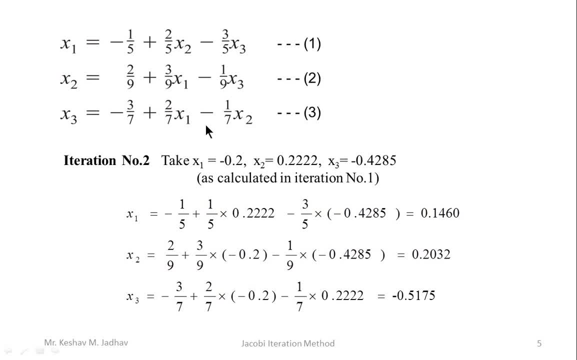 x2 as 0.2032.. Let us take third equation. In third equation also, we have to use values of x1 and x3.. In third equation also, we have to put these values of x1, x2, x3 so that we will get new. 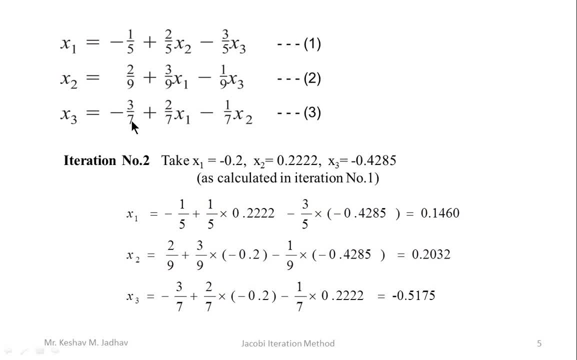 approximation for x3.. So here x3 is equal to minus 3 by 7. plus 2 by 7 into x1 is minus 0.2, minus 1 by 7 into x2 is 0.2222.. So if you put x1 is equal to minus 0.2 and x2 is equal to 0.2222,. 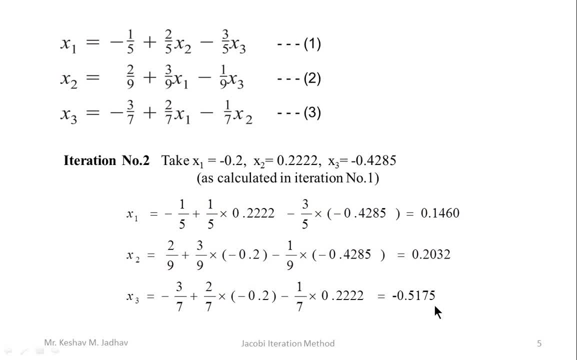 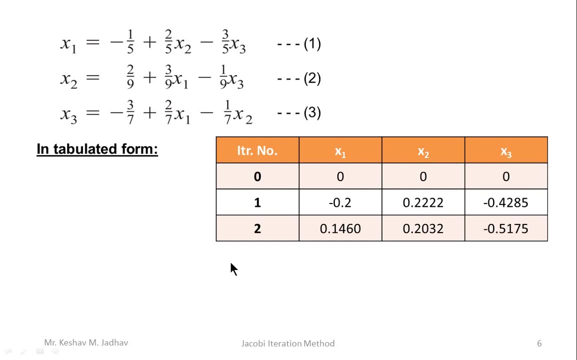 we will get new approximation for x3 as minus 0.5175.. So here we have to use values of x1, x2, x3 or next approximation value for x1,, x2, x3.. So we can write answer in tabulated form. So here we can write the values which are given in. 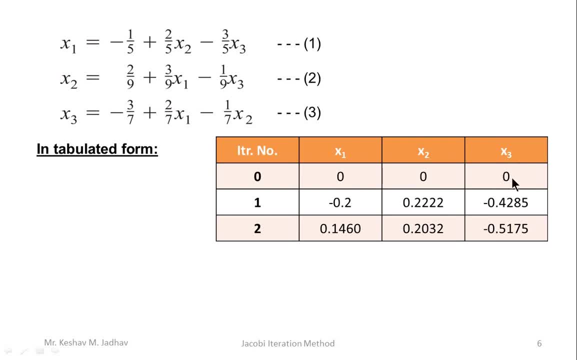 the example. So initial values of x1, x2, x3 are given as 0, 0, 0. So we can write here: So by using these initial values from these equations we will get new values of x1, x2, x3. 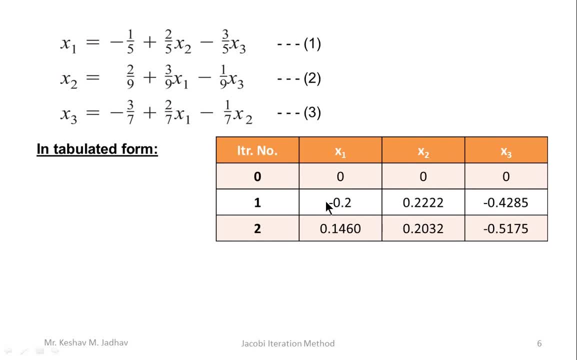 These are the values which we have got in iteration number 1.. Now, by putting these values of x1, x2, x3 in these equations, we will get second iteration values for x1, x2, x3.. Now, by putting these, 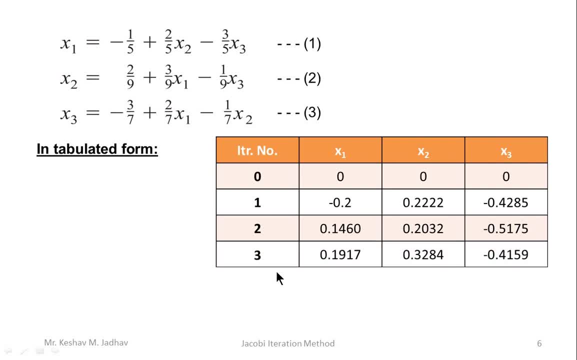 values of x1, x2, x3 in these three equations we will get values of x1, x2, x3 for third iteration. If we put third iteration values in these equations, then we will get values for fourth iteration.